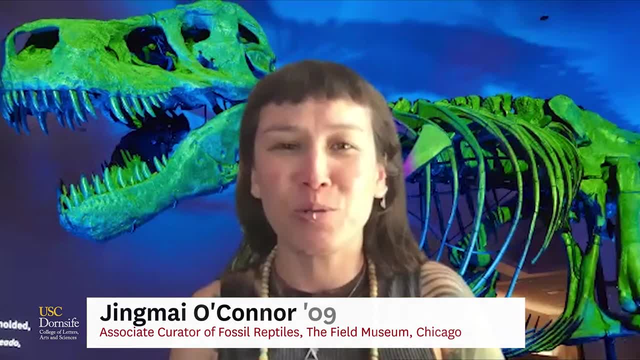 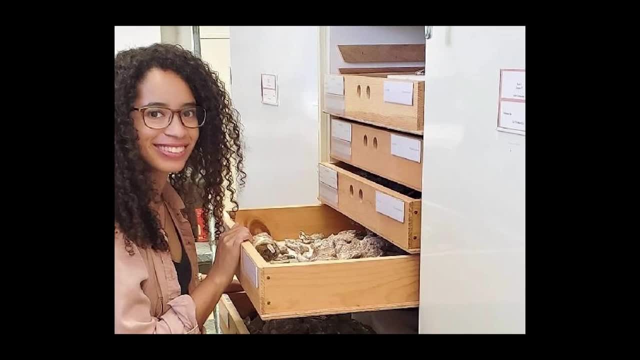 finding fossils in Mongolia, getting to go to conferences in Crete or studying collections in the Berlin Natural History Museum. My favorite part about doing paleontology is having the privilege of being able to handle and interact with fossils that are so incredibly old, from animals that existed before humans were. 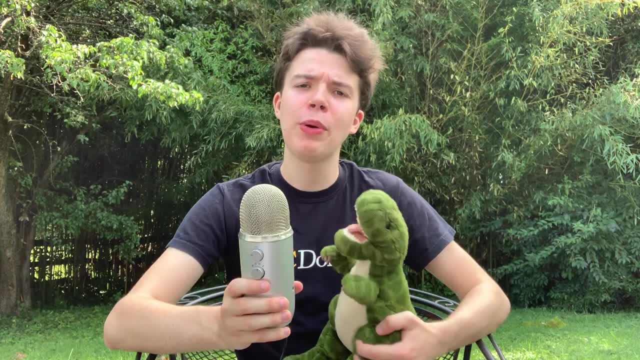 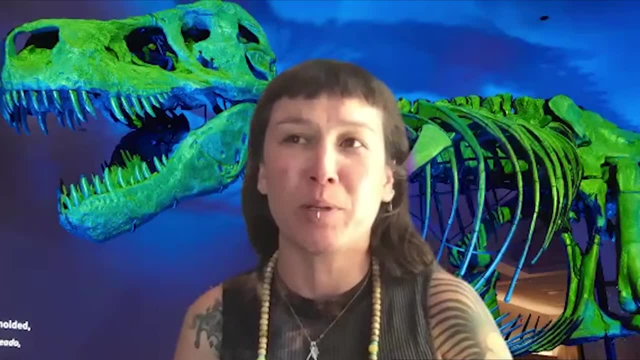 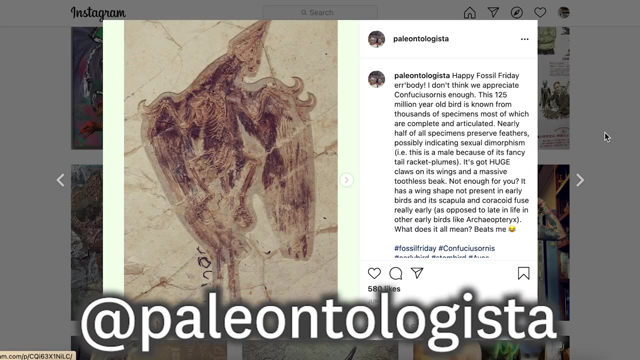 even a thought in evolution. Whoa Part of paleontology is communicating the knowledge that you gain about ancient life. So how do these Trojans share their studies with the community? Facebook and Instagram. and every Fossil Friday, I share a cool picture of a fossil and you know some interesting facts about it. 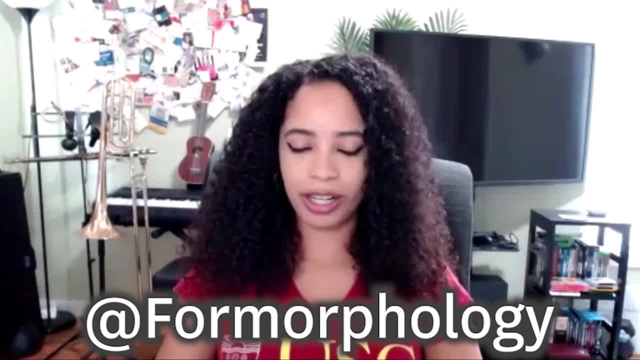 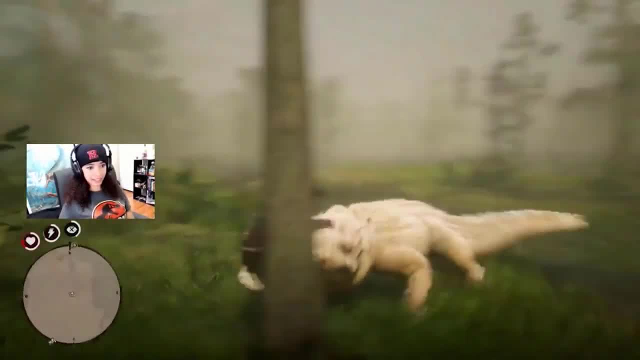 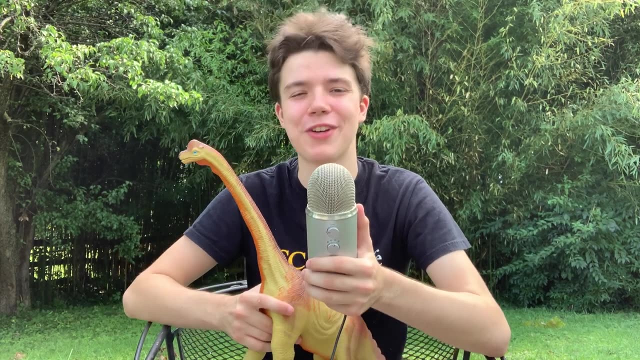 I am super active on Twitter. I share science memes. I'm also active on Twitch. I pretty much play games with a paleo twist. You can also find them in classrooms and at community events teaching about fossils. So now that we've gotten a peek at the world of paleontologists. 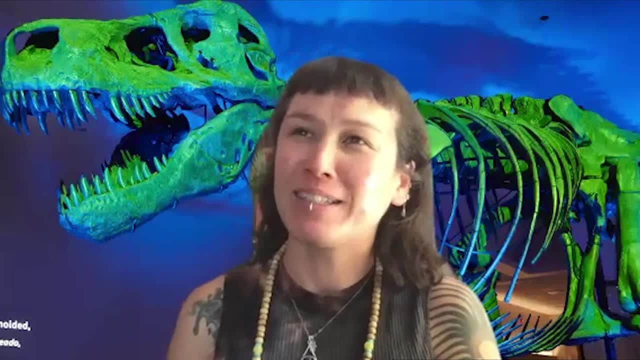 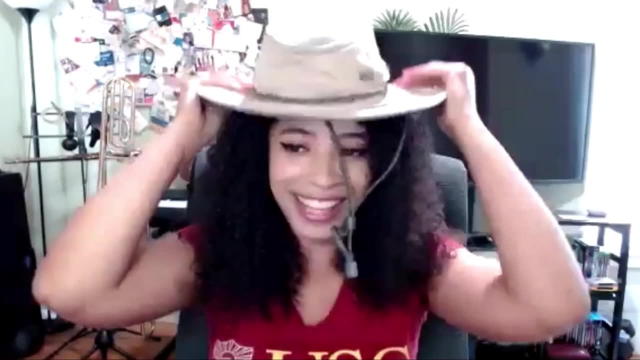 let's address some of the myths. I think the most obvious myth is that most paleontologists either look like Indiana Jones or they look like some old bearded guy wearing a hat. that looks like this. That does exist, but it's not just that. 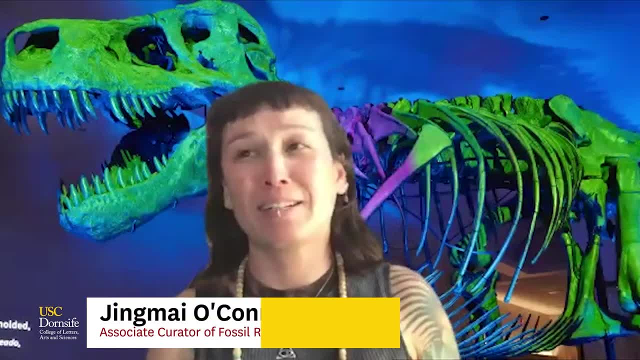 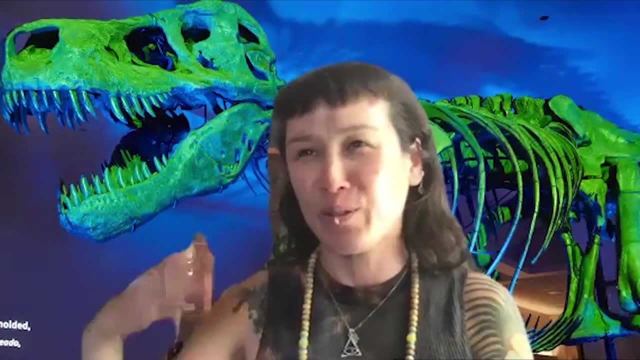 Paleontologists come in all shapes and sizes. Biggest myth is that dinosaurs are extinct. They're not extinct. So one group of dinosaurs managed to survive this end-Cretaceous mass extinction. If you look out your window and you see a bird, that's a dinosaur. 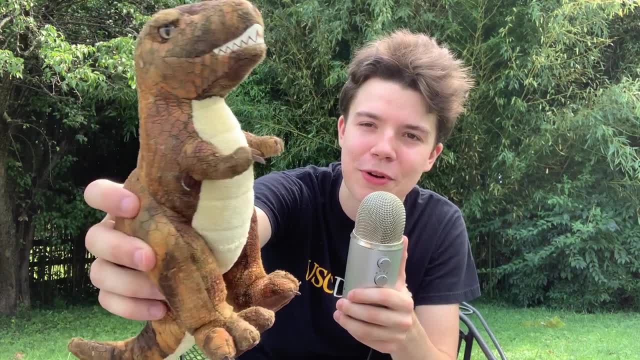 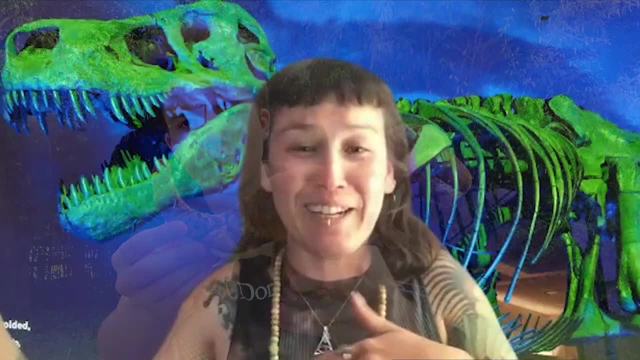 And I just had to ask: how accurate is this Tyrannosaurus rex plushie? Well, one thing we definitely know is that you know, their tails didn't drag on the ground. I mean, it won't stand up if you put the tail in the air. 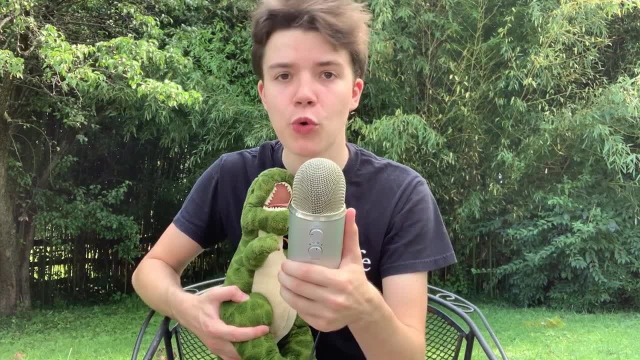 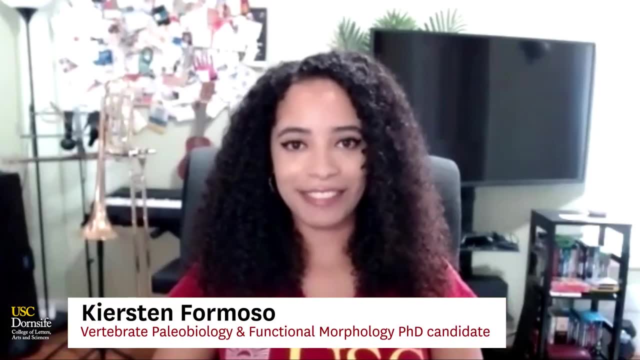 So they have to put the tail dragging down. So now onto the question we are all dying to know: Could we make a real life Jurassic Park today? No, we cannot. DNA has a very, very small half-life, A half-life that is well, well, well under when dinosaurs last existed on the planet. 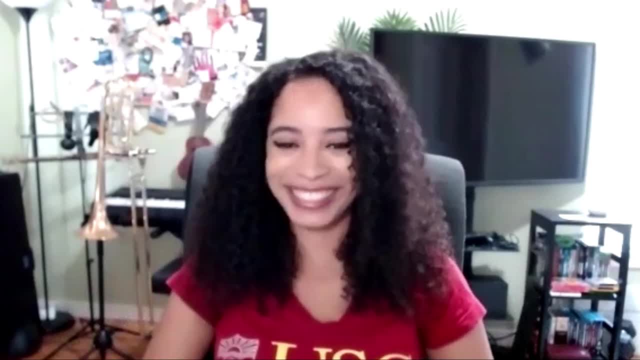 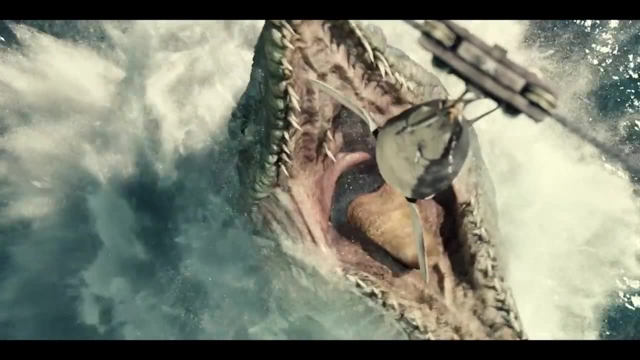 It makes me just as sad as it makes you. I promise I would love to like paddleboard over a Mosasaur, you know, assuming it doesn't like eat me. Now that we've solved some paleontology myths, what is some advice for you? loyal viewer.